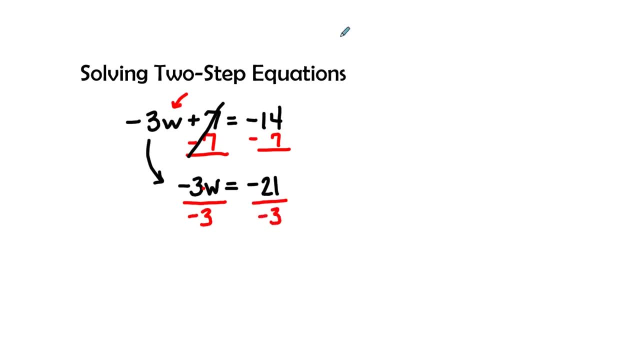 on both sides. So this will give me my negative 3 divided by a negative. 3 will give me my w by itself, and negative 21 divided by a negative 3.. Negative and a negative is a positive, and 21 divided by 3 is a positive 7.. So let's go ahead and check our work. 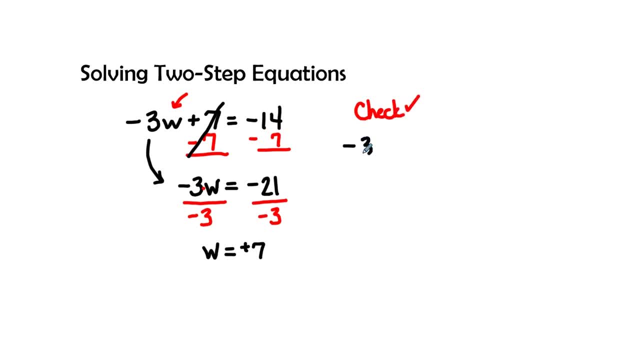 It's always good to check your work. Let's rewrite our equation, replacing the variable with the parentheses, so I can put in the positive 7, and it's going to equal a negative 14.. So here we go. Here's my positive 7.. So, negative 3. 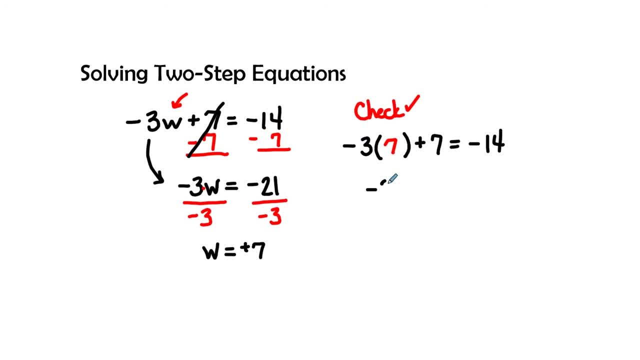 times 7 is a negative. 21 plus 7, and I'm going to go ahead and bring that down- is equal to a negative 14.. Negative 21 plus 7 is going to give me that negative 14.. So I know my. 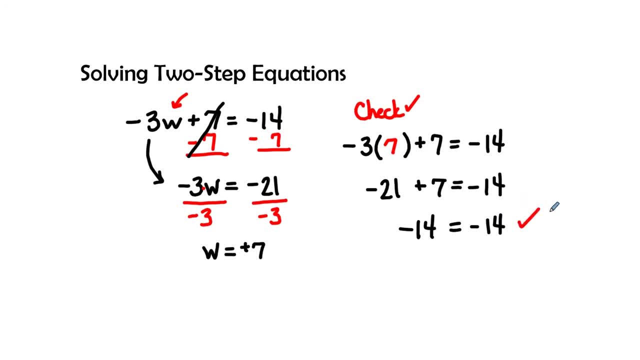 answer is absolutely correct. Let's try one more example. Let's go ahead and erase what we have here. So we're always remembering that we need to isolate our variable. We do that by inverse operations. So our second example is: let's do this in, let's do this in black. 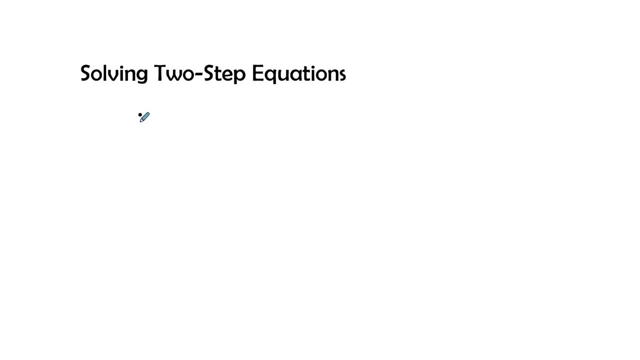 so we can accent our steps. in red, 16, minus 7m equals 30. So here we go. This 16, is really a positive 16. So it's attached to the variable by a positive 16.. Also this: 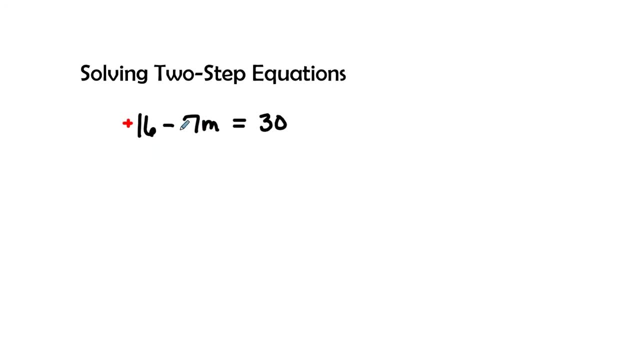 negative 7, is attached through multiplication as well, and so I'm going to put my multiplication sign just there just to remind me. but how I'm going to get rid of this positive 16,? I'm going to go ahead and do an. 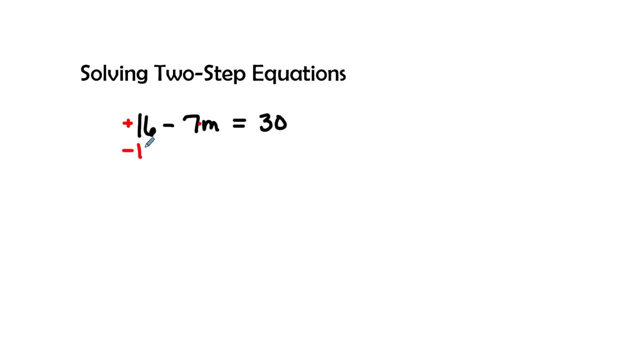 16. So I'm going to. its inverse is a negative 16.. So I'm going to add a negative 16 to both sides of the equation. So this gives me zero. I'm going to go ahead and bring down my negative 7m.